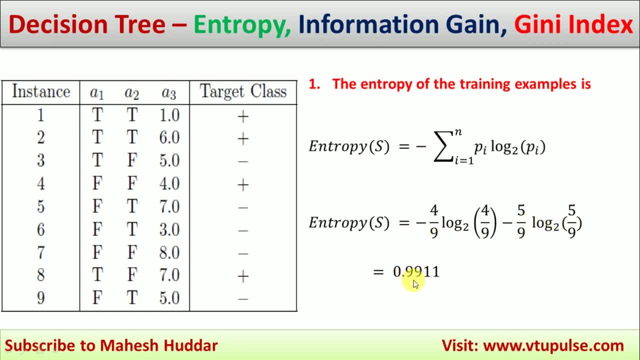 If you solve this equation, you will get the entropy as 0.99.. Here, if you want to know how to find the logarithm with base 2, you can use this equation: That is, log of a to the base 2, that is equivalent to logarithm of a divided by logarithm of 2.. 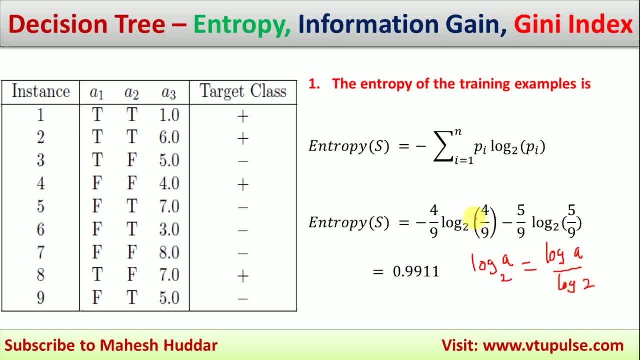 So this is the equation you can use to find the logarithm. with any value, the base is equivalent to 2 in that case. So we understood how to find the logarithm with base 2.. Now we are going to calculate the entropy here. 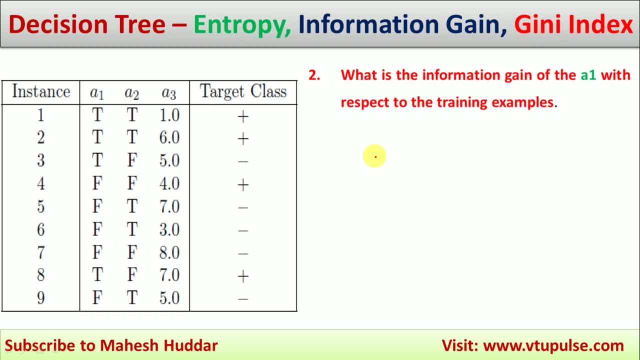 Now we try to find the information gain of attribute A1 here. In this case, A1 has two possibilities: One is true and another one is false in this case. So first we need to find the entropy of true examples and entropy of false examples. 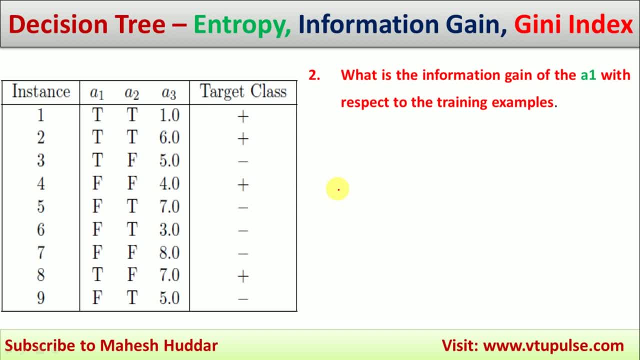 We have already calculated the entropy of four data sets. So considering these three we can calculate the information gain of A1 here. So we know that the entropy of A1 is 0.99.. The entropy formula is minus summation of pi, log pi to the base 2.. 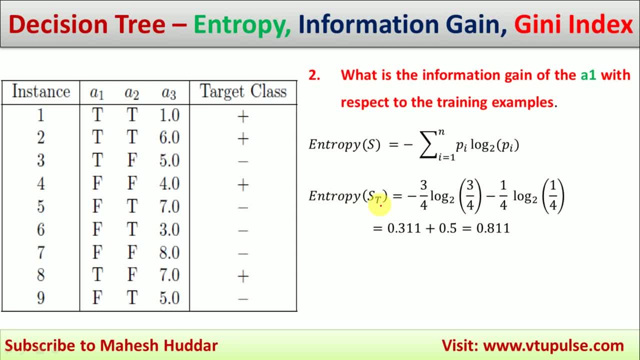 The entropy of the data set where the A1 is equivalent to true is always equivalent to minus 3 by 4.. That is if you consider there are 1, 2, 3, 4.. Four true examples are there. 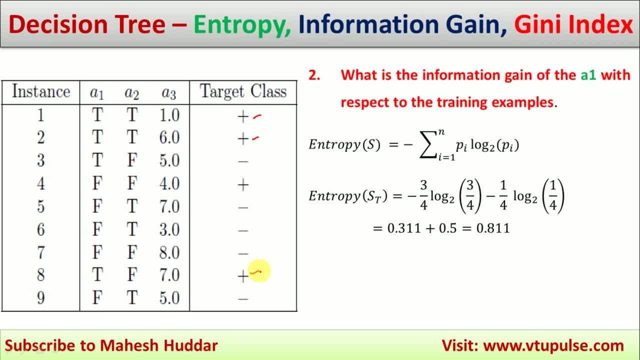 Out of that, 1,, 2 and 3 are positive examples and 1 is negative example. So the probability, Probability of positive examples within true that is 3 by 4, log 3 by 4 to the base 2,. 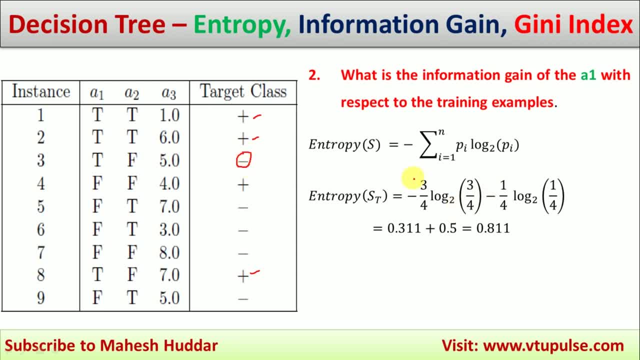 minus negative examples. this is the only negative example we have here. that is 1 by 4. log 1 by 4 to the base 2.. And if you solve this equation you will get. the entropy of true examples is 0.811.. 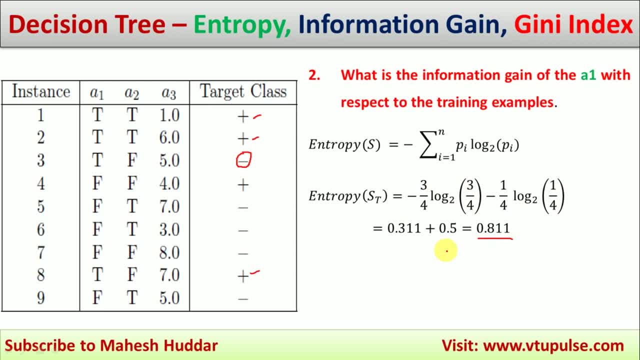 Similarly, we need to find the entropy of false examples. There are 1,, 2,, 3,, 4, 5.. 5 false examples are there. So out of 5 false examples we can see here, this is the positive example. negative, negative, negative and negative. 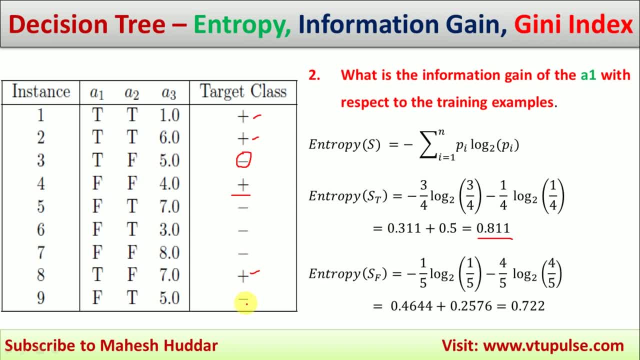 So 1 is positive and remaining 4 are negative examples here. So the entropy of Sf, that is the data set when the false examples are there, which is equivalent to minus 1 by 5.. That is 1 positive example is there out of 5, log 1 by 5 to the base: 2, minus 4 negative examples are there. 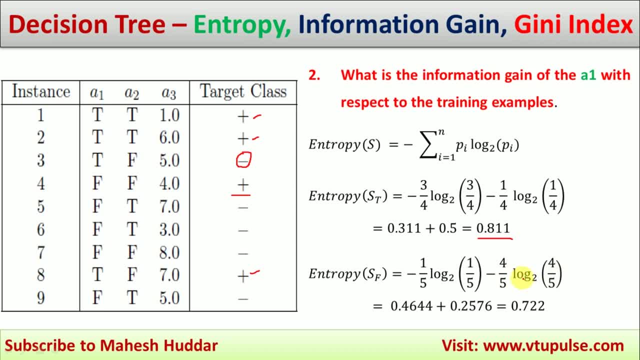 So 4 by 5.. Log 4 by 5 to the base 2 here And if you solve it you will get the entropy of false examples is 0.722.. Now, using these two and the entropy of false data set, we can calculate the information gain of A1 here. 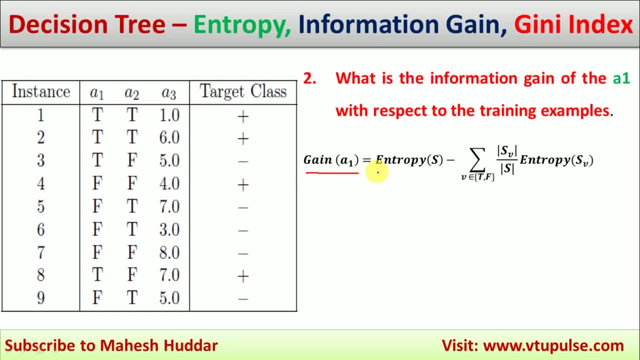 That is, the gain of A1 is always equivalent to the entropy of false data set minus the entropy of individual data set should be multiplied by their the proportionate values, That is, the proportionate values. The proportionate values- proportionate true examples multiplied by entropy of true examples. proportionate false examples multiplied by entropy of false examples, that is equivalent to entropy of S, as it is minus 4 by 9.. 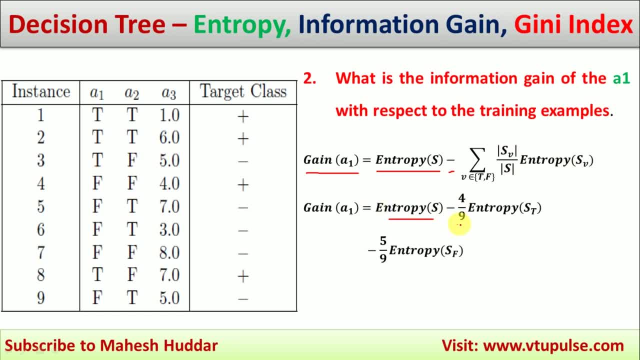 That is, there are 4 true examples are there out of 9, that is 4 by 9. here, entropy of the true examples minus 5 by 9, that is proportionate of false examples multiplied by entropy of false examples. 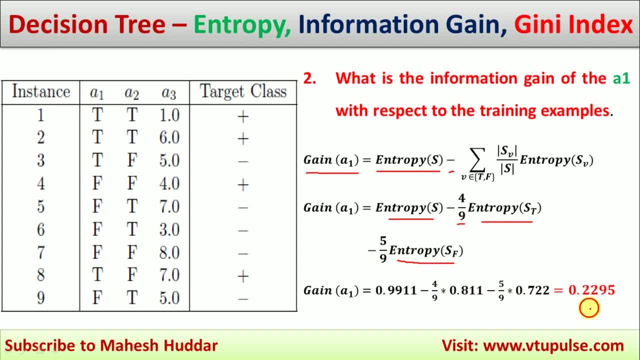 examples. put all the values in this particular equation you will get. the entropy is equivalent to. that is sorry. the information gain is equivalent to 0.2295 in this case. so the information gain of a1 is equivalent to 0.2295. similarly, we will try to identify or find the. 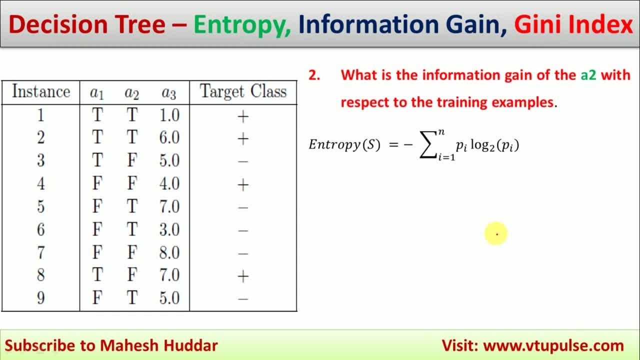 information gain of a2. here again we need to find the entropy of possible values of a2. there are two possible values, again true and false. now the entropy of true examples is: there are five true examples are there? 1, 2, 3, 4, 5 out of 5 you can see here the first and second one are true and 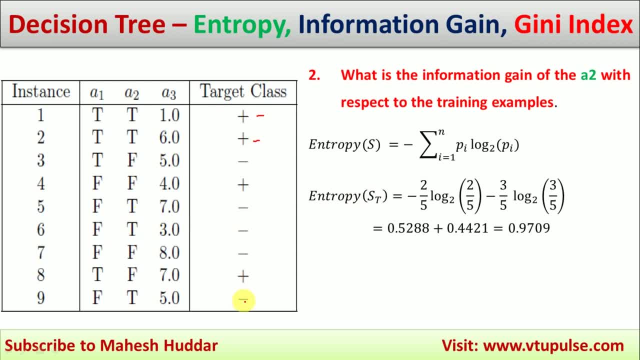 remaining 1, 2 and 3 are negative examples here. okay, so you can say that minus 2 by 5, log 2 by 5, to the base 2, that is positive examples. minus 3 by 5, log 3 by 5, log 2 by 3 to the plus larger the interval between 1 and 2, so and will give you 2 x del Aloha. 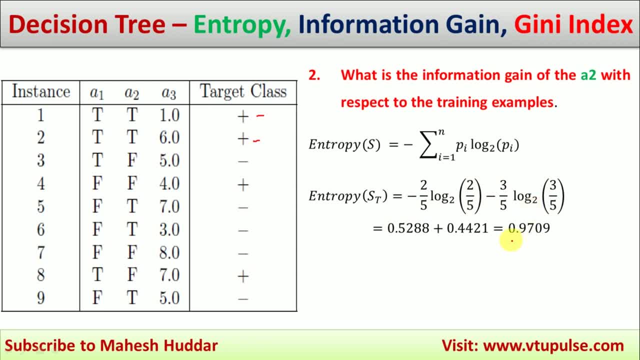 3 x del Aloha, so for a 3 so and will give you 2 x del Aloha. so to say that log 2 x del Aloha, so理 R1 1 for by 5 to the base 2. that is negative examples and if you solve it you will get the entropy as. 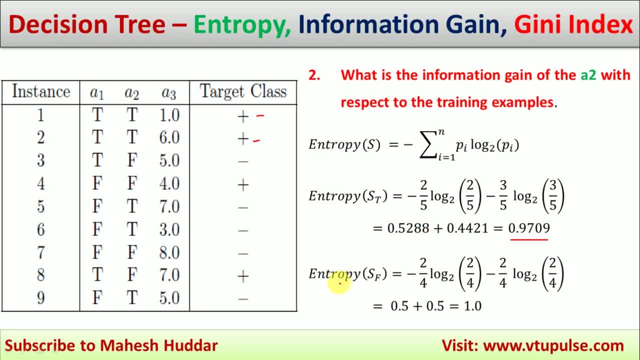 0.9709. similarly, we will calculate the entropy of false examples: 1, 2, 3, 4. four false examples are there. out of that, first one is negative, second one is positive, third one is negative and fourth one is positive. so two positive and two negative examples are there, so entropy is equivalent to: 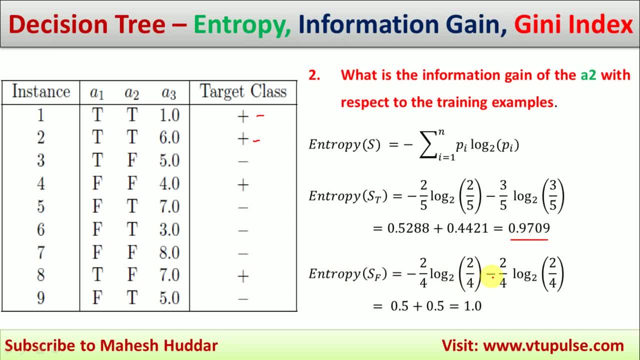 minus 2 by 4, log 2 by 4 to the base 2, minus 2 by 4, log 2 by 4 to the base 2, and if you solve it you will get the entropy as 1.0. now we will use the gain formulae to calculate the gain of a2 here. 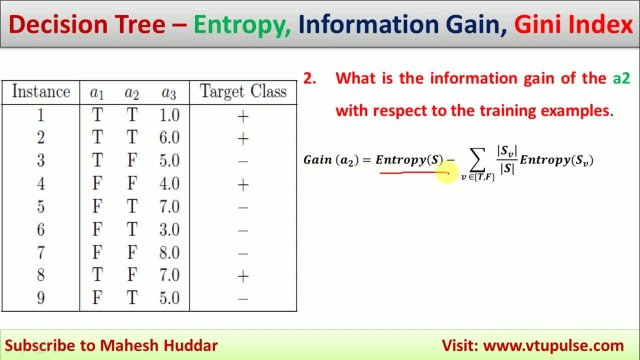 the gain of a2 is equivalent to entropy of whole data set, minus proportionate of positive examples. this is a proportionate of true examples- entropy of true- minus proportionate of false examples- entropy of false examples. so that is what is written here, so v is equivalent to either true: 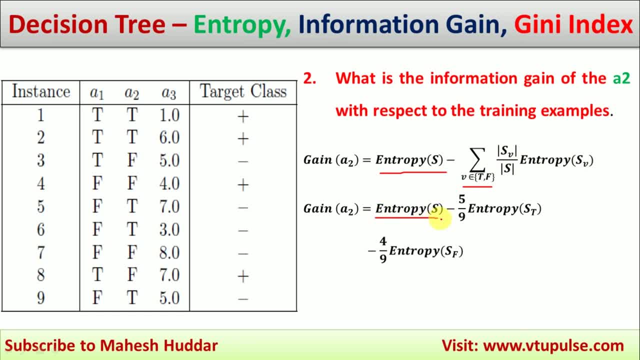 and false in this case. that is entropy of s minus 5 by 9. that is 5 times true. examples are there out of 9. entropy of true example: 4 times false. examples are there. so 4 by 9. entropy of false. here. put all the values, you will get the gain as 0.0072 in this case. so gain of a2 is 0.0072. 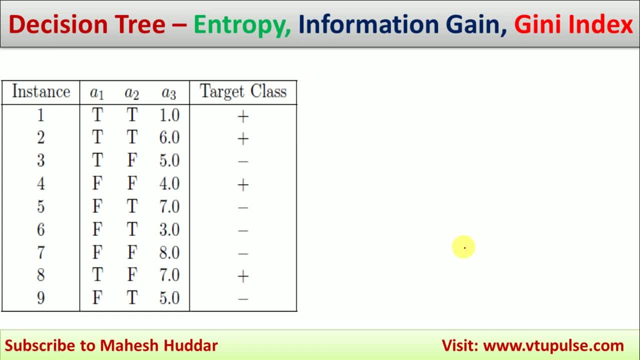 now we will try to find the Gini index of these two attributes, that is, a1 and a2. so before you calculate the Gini index, first you need to calculate the Gini of those particular attributes and then you can go ahead with Gini index. so Gini is always equivalent to 1 minus summation of. 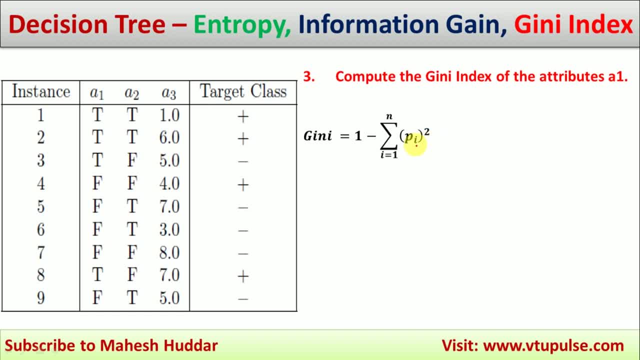 pi square, where pi is the probability of ith class. ith class in. in that case now Gini of t. first we will try to calculate the Gini of true examples only, and then we calculate the Gini of false examples, and then we will go with the Gini index. so Gini of true examples is: 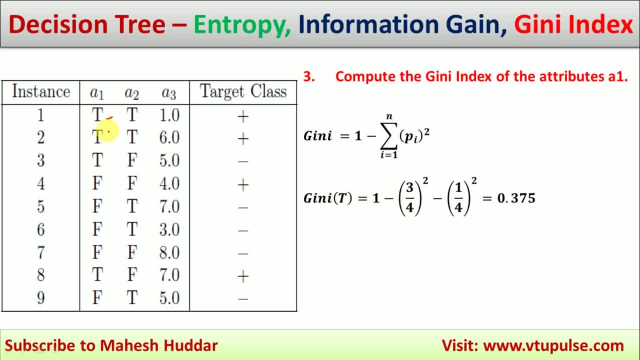 equivalent to 1 minus. so there are totally 4 true examples are there. you can see here, out of 4, 1, 2 and 3 are the positive and this is the only negative example we have here. so 1 minus 3 by 4. 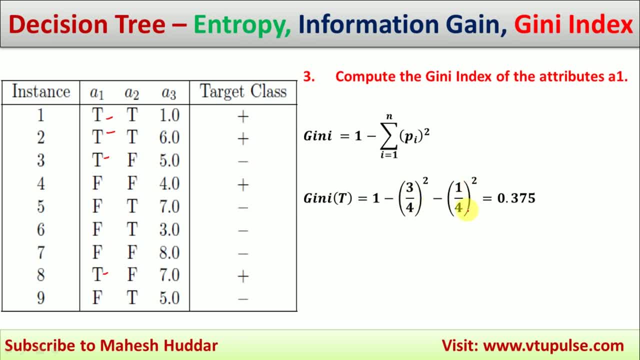 probability of positive examples minus 1 by 4, that is probability of negative examples, which is equivalent to 0.375. similarly, we will try to find the Gini of false examples, that is 1 minus probability of positive examples, minus probability of negative examples, within false. so totally we. 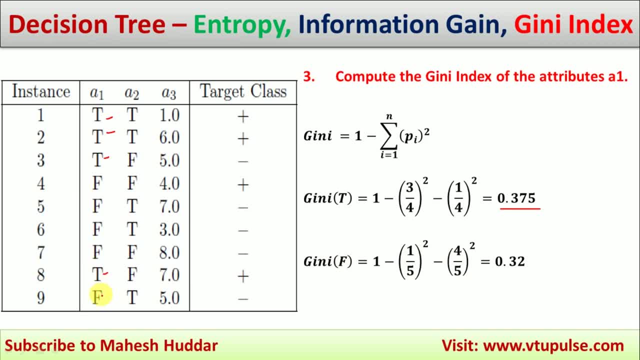 have one, two, three, four, five false examples are there. out of that, one is true and remaining all are. one is positive and remaining all are negative examples here. so 1 minus 1 by 5, that is probability of positive examples, minus 4 by 5, that is probability of negative examples. and if you 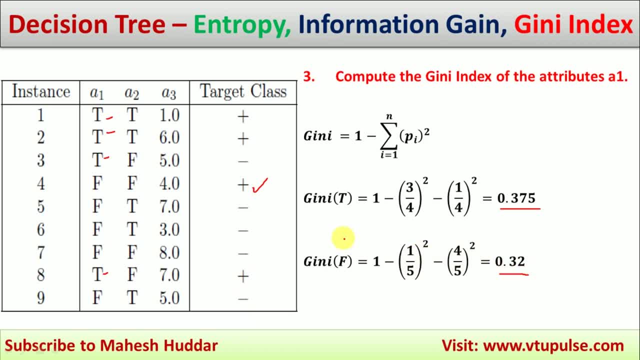 solve it, you will get 0.32 as the answer in this case. so once you calculate the Gini of true and false, now we need to calculate the Gini index. the Gini index of a1 is equivalent to the proportionate of true examples multiplied by Gini of true examples plus proportionate of false examples. 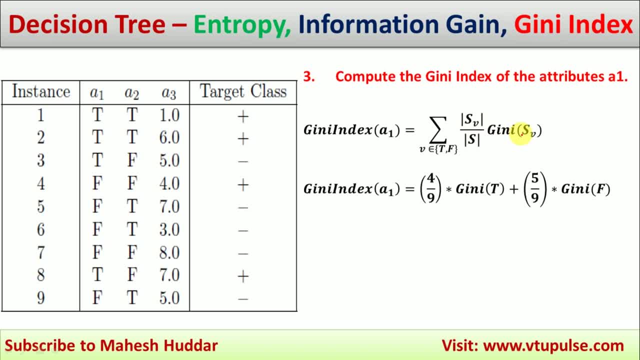 multiplied by Gini of false examples here, that is 4 by 9. that is 4 times true examples are there out of 9 Gini of true, 5 false examples are there. that is 5 by 9 multiplied by Gini of f, in this case put. 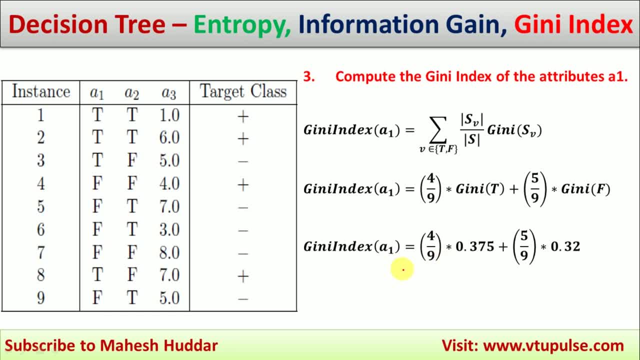 all the values, what you have calculated in the previous step, you will get. the Gini index of a1 is 4 4- 4 in this case. similarly, we try to calculate the Gini index of a2 before that we need to calculate the Gini of true and false, because a2 also has the two possibilities, true and false- in 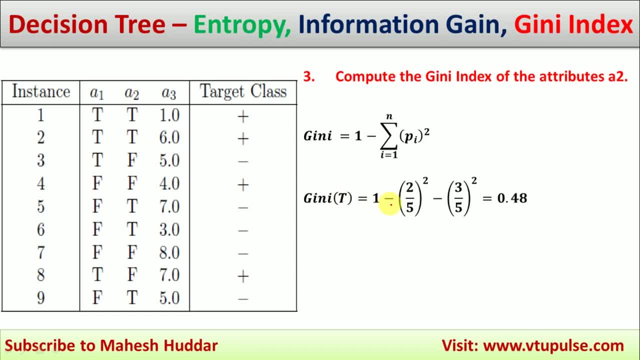 this case. so Gini of true is equivalent to 1, minus the proportionate of positive and negative examples within true examples. so 1, 2, 3, 4, 5, 5 true examples are there. out of that, 1, 2 are positive remaining. 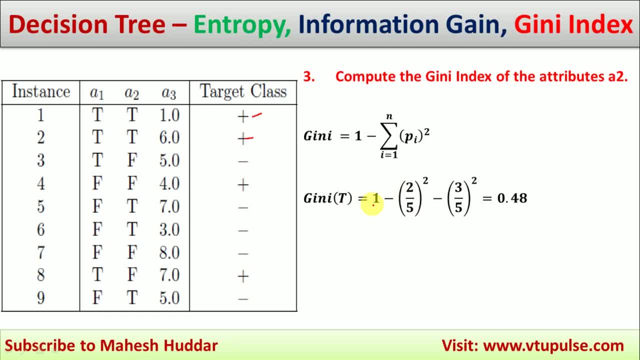 1, 2, 3 are negative here. so 1 minus 2 by 5 bracket square, that is the proportionate of positive examples. minus 3 by 5 bracket square, that is proportion of negative examples, which is equivalent to 0.48. similarly, Gini of f, which is equivalent to 1 minus. first we need to know how many false. 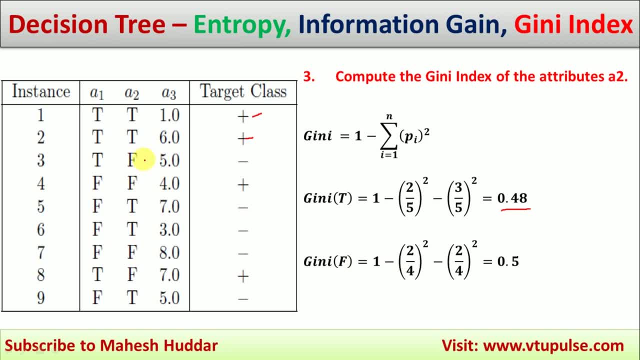 examples are there. one, two, three, four, four false examples are there. first one is negative, second one is positive, third one is negative, fourth one is positive. so two are positive, two are negative, hence 1 minus 2 by 4 bracket square, minus 2 by 4 bracket square, which is 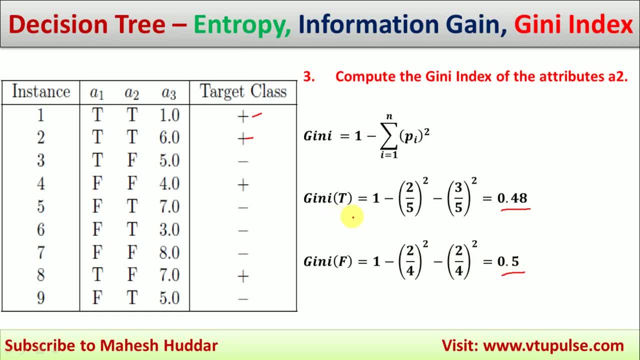 equivalent to 0.5 in this case. so, finally, the Gini index of a2 is equivalent to the proportionate of true examples multiplied by Gini index of Gini of true, plus proportionate of false examples multiplied by the Gini of false. here so put all the values which is calculated in the previous 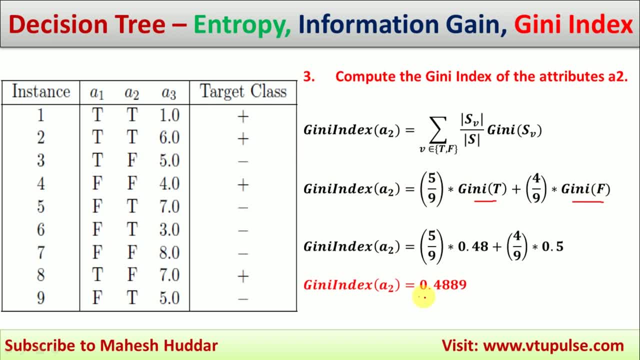 step, you will get. the Gini index of a2 is equivalent to 0.4 889 in this case. so we understood how to calculate the entropy, how to calculate the gain of a1 and a2, as well as Gini index of a1 and a2. now we need to understand how to select the splitting attribute. 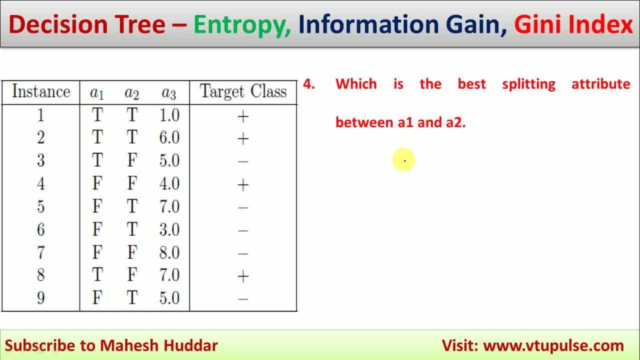 based on these things, now we know that the gain of a1 is equivalent to 0.2295. that is calculated in the previous step. the gain of a2 is equivalent to 0.0072. in this case, the gain of a1 is equivalent.